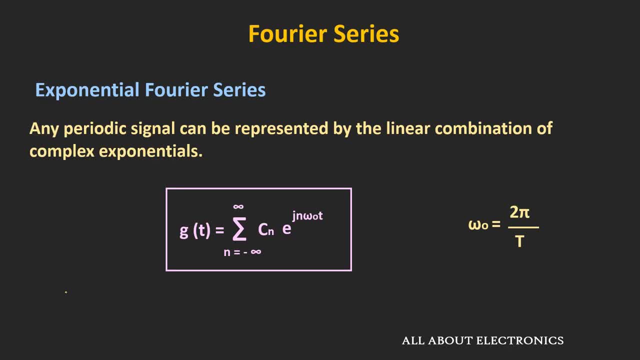 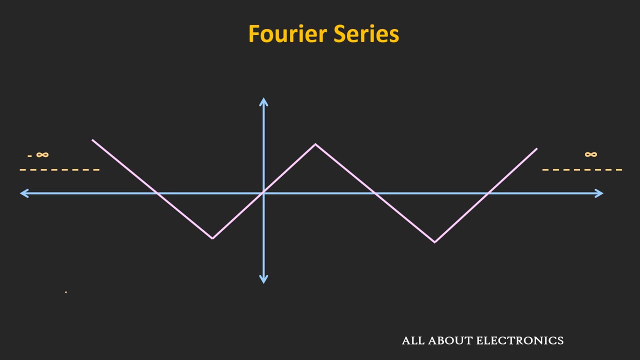 useful. So so far in the earlier videos we had seen that using this Fourier series we can find the frequency spectra of any periodic signal. The periodic signal repeats itself after some finite time and it exists from minus infinity to plus infinity. But all the practical signals are the aperiodic. 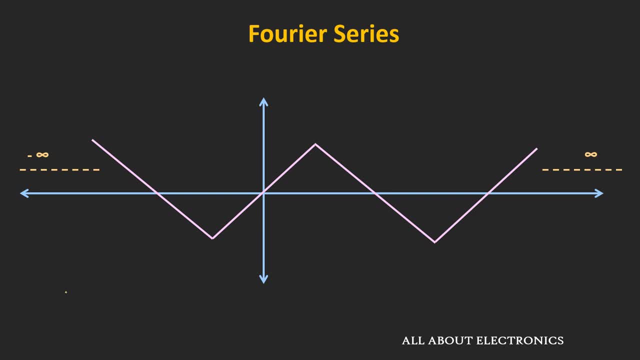 Because they start at some finite time and they also end at the particular time. For example, if we take the case of the speech signal, then it exists only for the finite duration. That means almost all practical signals are the aperiodic signal. 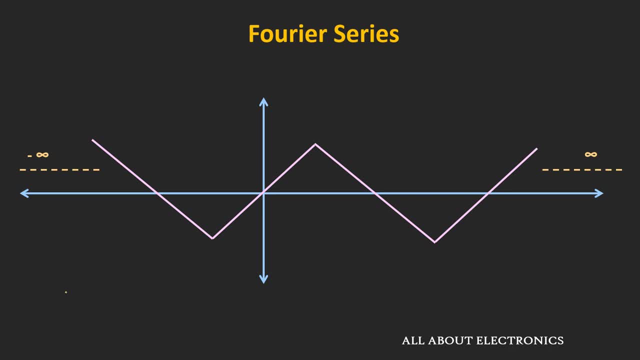 And for such aperiodic signal we can find the frequency spectra using the Fourier transform. So let's say we have this aperiodic signal and we want to find the frequency spectra of this aperiodic signal, And let's say this signal exists from the time t1 to t2.. 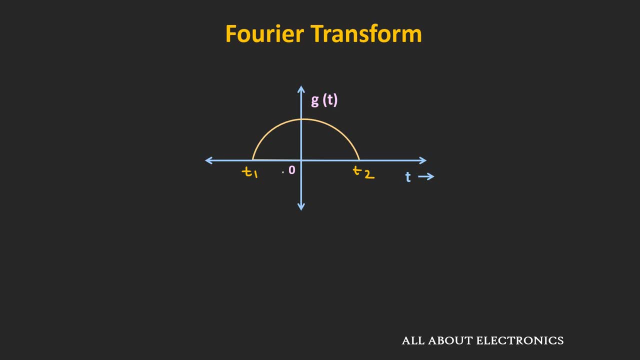 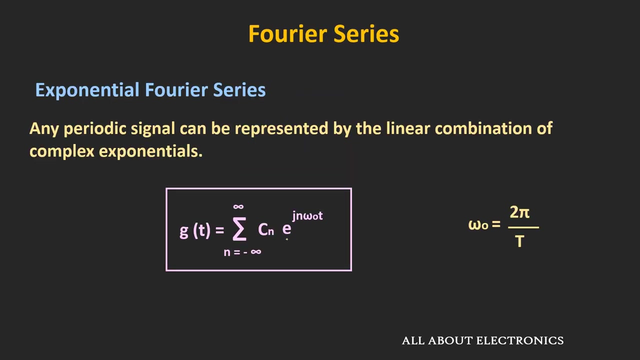 So using the generalized expression of the Fourier transform we can find the frequency spectra of this aperiodic signal. But to understand this Fourier transform little bit in detail, let's start with the exponential Fourier series And if we apply certain limiting process then this aperiodic signal can be represented. 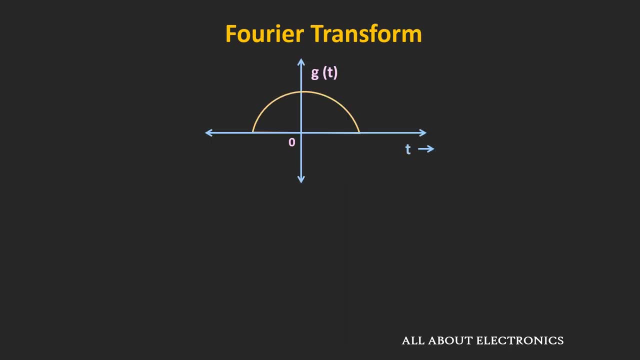 as the summation of these complex exponentials. So for that let's define the new periodic signal from this aperiodic signal, So, as you can see, this new signal g repeat itself after the one time period. t is the periodic signal. 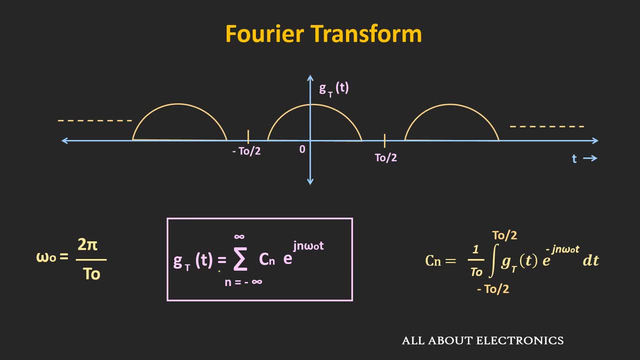 So we can represent this signal by the summation of the complex exponentials, And here the contribution of each complex exponential can be found using this expression. Now, here, if you observe, this periodic signal is integrated over the one time period, right. 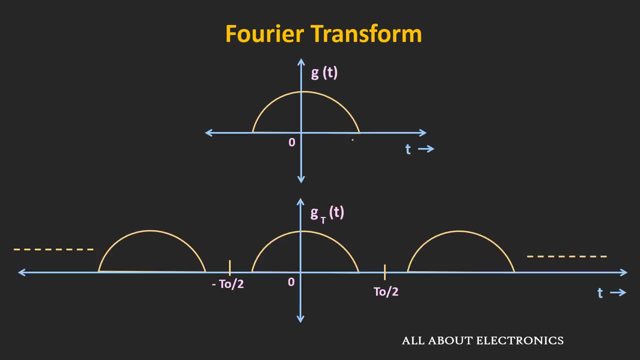 But instead of integrating this periodic signal, if we integrate this aperiodic signal from minus infinity to plus infinity, then it will give us the same result, right? So we can write this Cn as 1 by t0 integration gt e to the power minus j times nω0t dt. 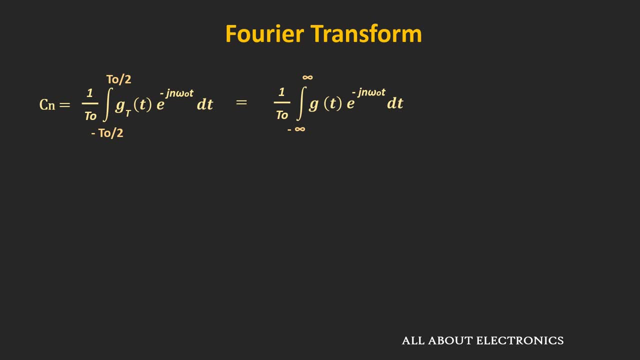 And using this expression we can find the coefficients at the different frequencies And let's say, for the given signal. these are the coefficients Now here, if we double the time period of this signal, that means if t0' is equal to. 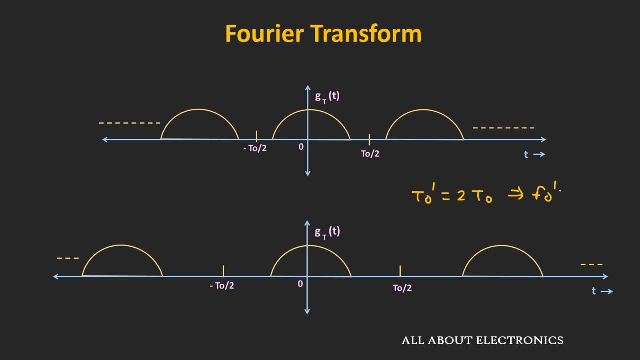 2 times t0, then the frequency will get 1⁄2.. So we can write this Cn as 1 by t0, integration gt of t e to the power minus j times nω0t dt, And using this expression we can find the coefficients at the different frequencies. 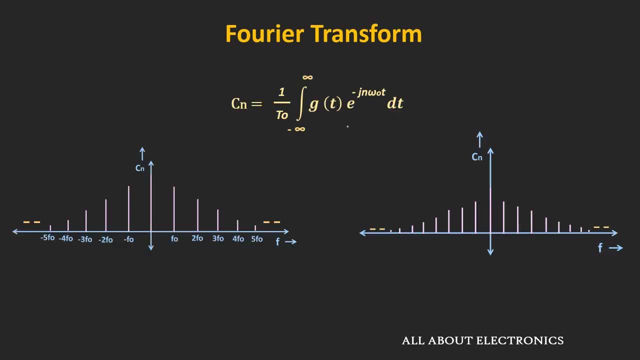 So we can write this Cn as 1 by t0 integration gt of t e to the power minus j times nω0t dt. And here, since the time period has been doubled, so the amplitude or the weightage of each coefficient will also reduce. 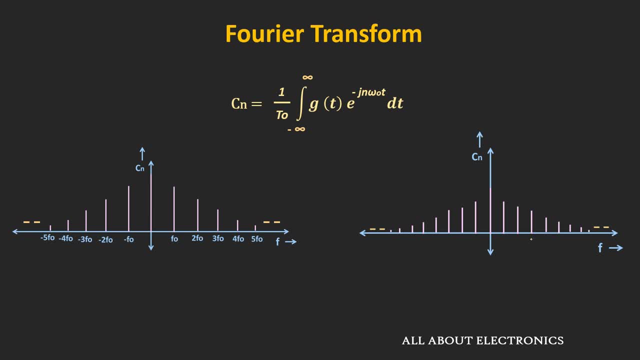 And as we increase the time period of the signal, then the spectral components will get closer and closer. Or in other words, we can say that the frequency spectrum will get denser And as this time period t0 tends to infinity, that means when the signal repeats itself. 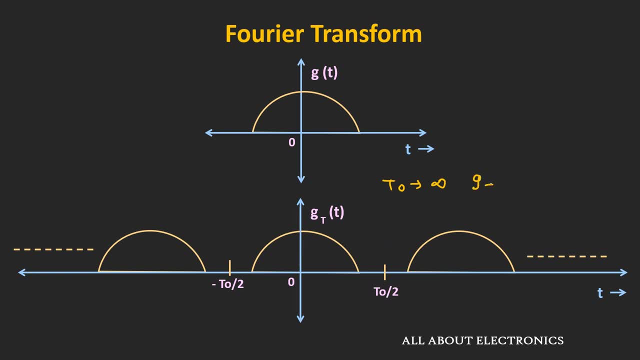 after the infinite time period. Then we can say that here this gt of t is equal to g of t. That means, as t0 tends to infinity, then the spectral components are no longer discrete. That means in that case we will get the continuous frequency spectrum. 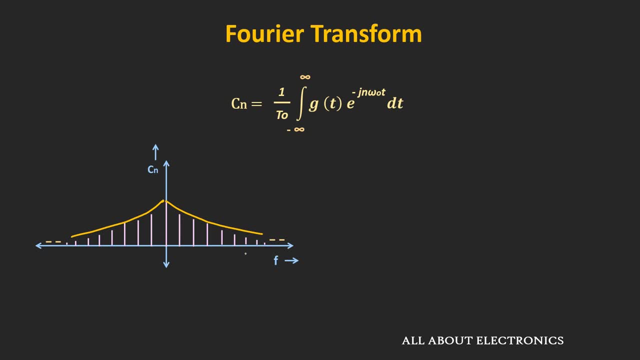 And now, since this frequency spectrum is continuous, so we cannot define the frequency components by this Cn. So this continuous frequency spectrum can be defined by the following expression: And this expression can be defined by the following expression: And this expression can be defined by the following expression: 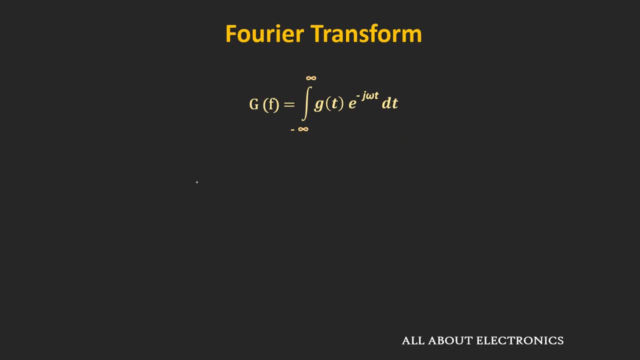 And this expression shows the Fourier transform of the signal g. That means if we take the Fourier transform of this signal g, then we will get the continuous function g in the frequency domain. So so far what we did. from this aperiodic signal we generated the new periodic signal. 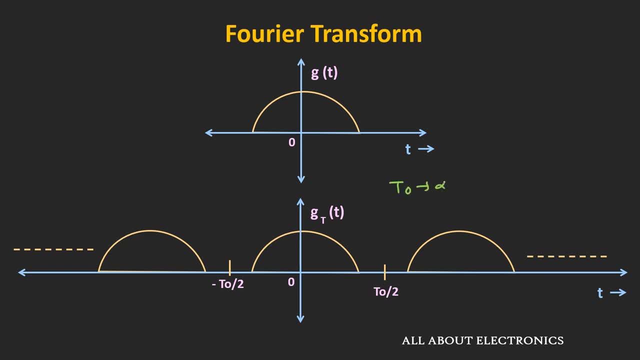 And for this periodic signal, by assuming t0 tends to infinity, we got the expression of the Fourier transform. Similarly, if we know the frequency spectrum, So if we know the frequency spectrum of any signal, then using the inverse Fourier transform, 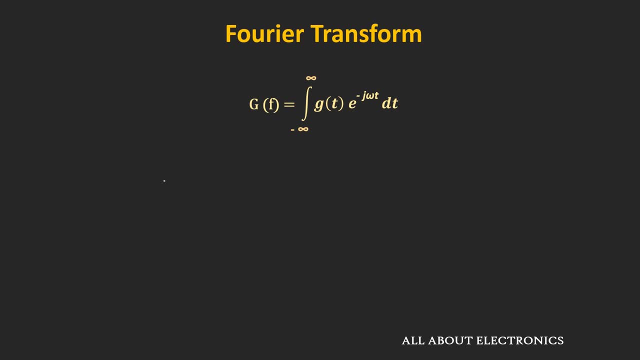 we can reconstruct that signal in the time domain. So this inverse Fourier transform can be given as integration: minus infinity to plus infinity, g, e to the power, j times ωt times df. So this expression shows the inverse Fourier transform. So now let's talk a little bit about this inverse Fourier transform. 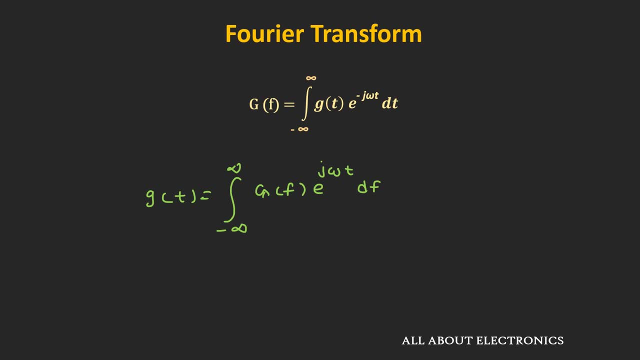 And to understand it we will use the following expression: So, as I said, if we have the periodic signal g, then it can be expressed as the linear combination of the complex exponentials, And here the weightage or the contribution of each component can be given by this expression. 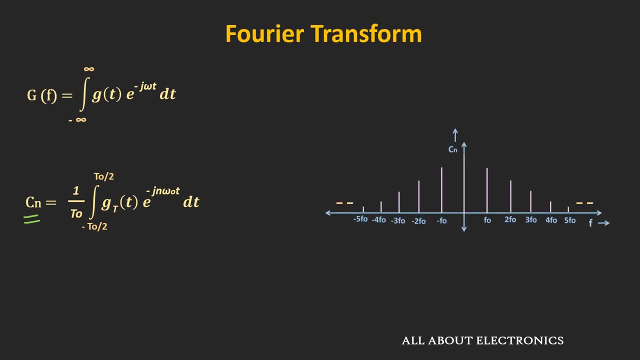 So here this Cn shows the frequency components of the signal g, while this expression shows the frequency spectrum of the aperiodic signal g. Now, as I said earlier, this Cn can be written as 1 by T0, integration minus infinity to infinity. 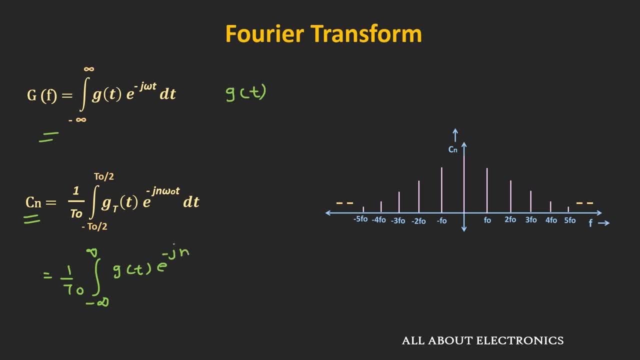 g times e to the power minus j times nΩt dt. So if we compare this expression with g, then we can write it as: Cn is equal to 1 by T0 times g. And here this expression shows the samples of the continuous function g which is taken. 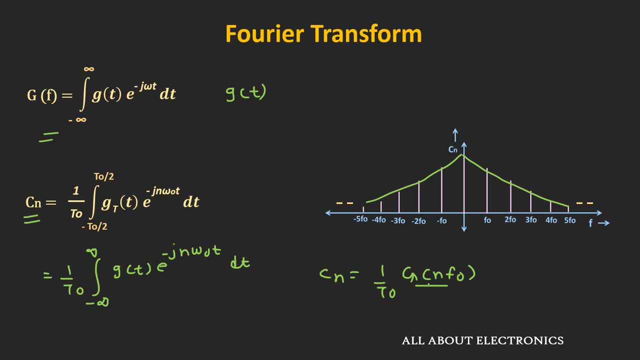 at the interval of f0. That means if we put the value of n is equal to 1, then we will get the value of C1, which is the sample of this function, g taken at the f0. And likewise, by putting the different values of n, we will get the sample of this function. 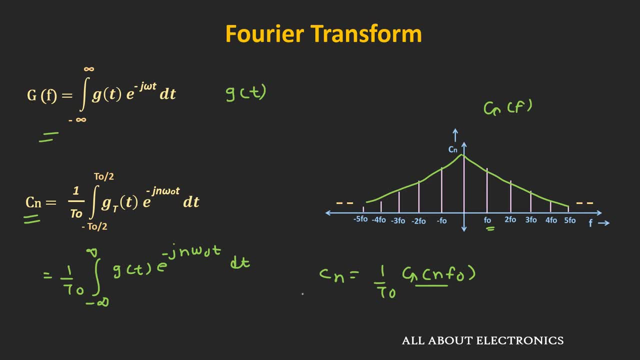 g at the different intervals. So now let's put this value of Cn in this summation. That means we can write this expression as: gt is equal to summation of n is equal to minus infinity. to plus infinity, 1 by T0 times g, times e to the power, j times. 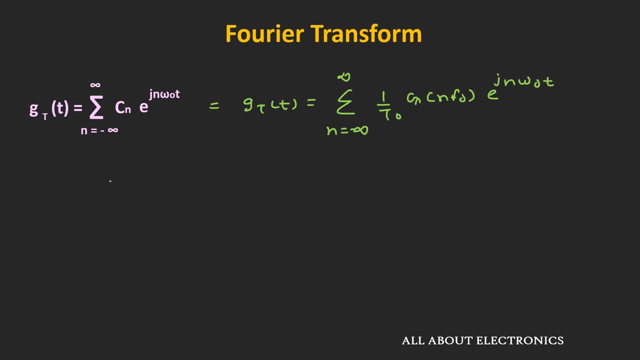 nΩt. Now here. as T0 tends to infinity, then we can say that this f0 tends to zero. And when this f0 tends to zero, we can write this expression as gt. then the more meaningful representation of this F0 is equal to ΔF. 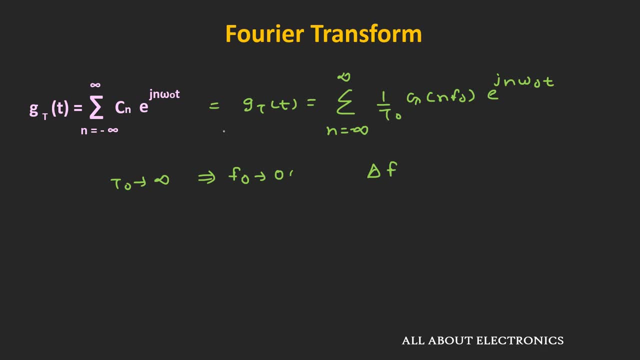 So, considering this, when this T0 tends to infinity, then we can write this expression as summation: n is equal to minus infinity to infinity, this ΔF times g and ΔF times e to the power j times n times this ω0 is equal to 2π times F0.. 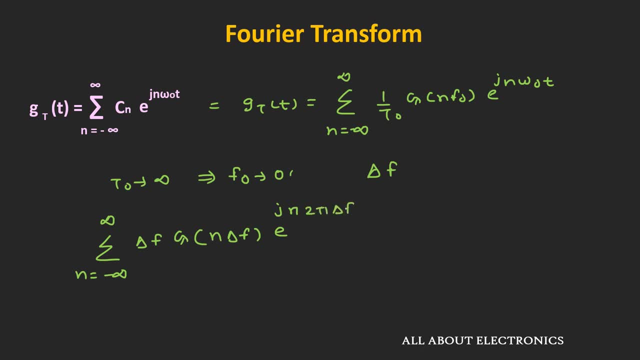 That means we can write it as 2π times ΔF times T. So this is the expression of this g when this T0 tends to infinity. And graphically, if we see this expansion, then this small segment represents the nΔF.